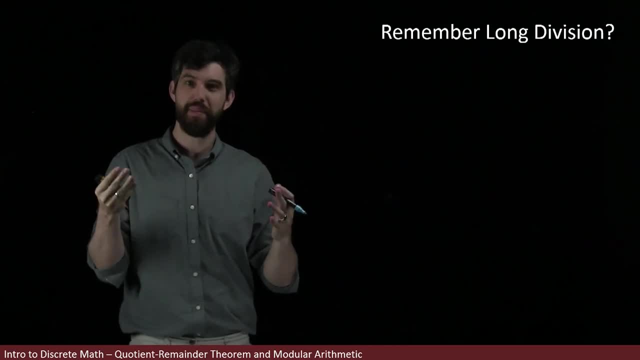 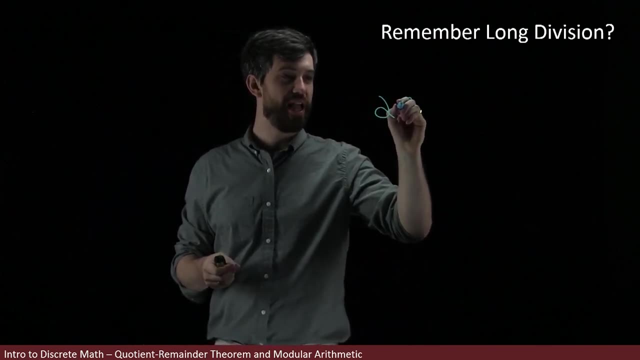 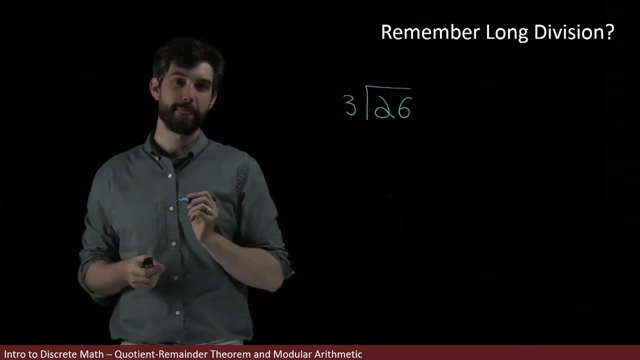 and make precise statements about it using all of our new mathematical terminology. So let's see an example that reminds us how this works. If I take some number like, say 26,, and then I want to divide it out by three, The way this worked is: you tried to take the 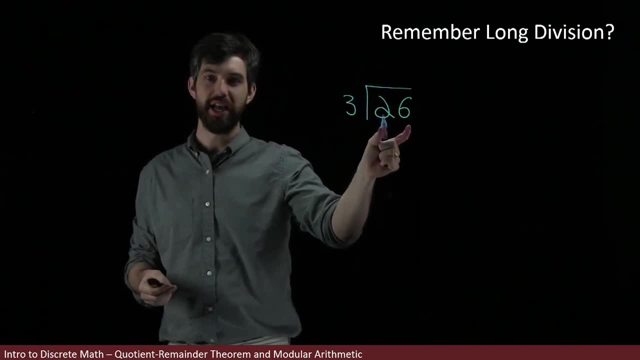 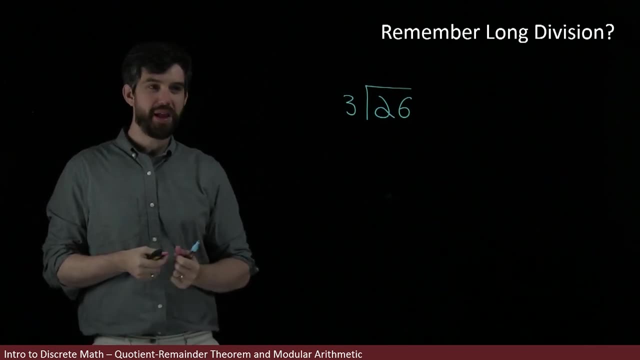 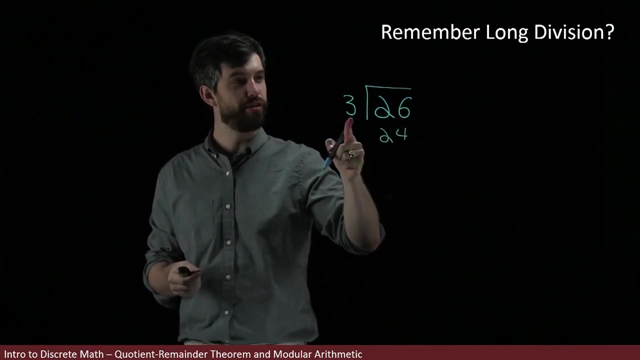 three and you chose some number that was as close to 26 as you could imagine but was divisible by three. So, for example, the number 24, I'm going to write that down- The number 24 has the property that three, and I wrote the other factor here. 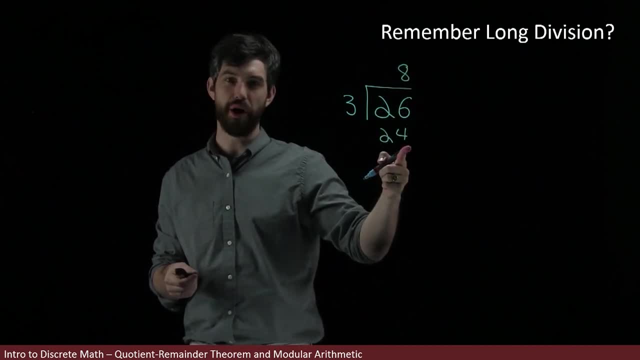 I'm going to write that down. The number 24 has the property that three- and I wrote the other factor here here- 3 times 8 was equal to the 24.. So in other words, this number that I'm putting down here, 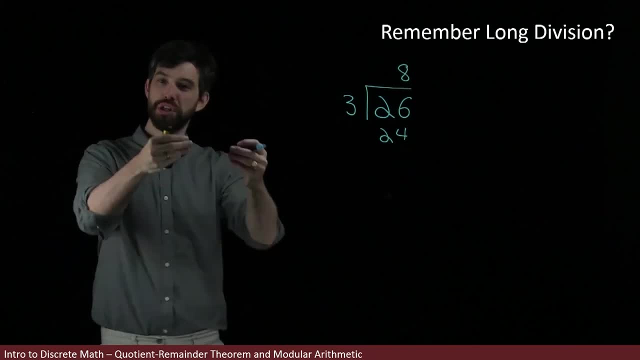 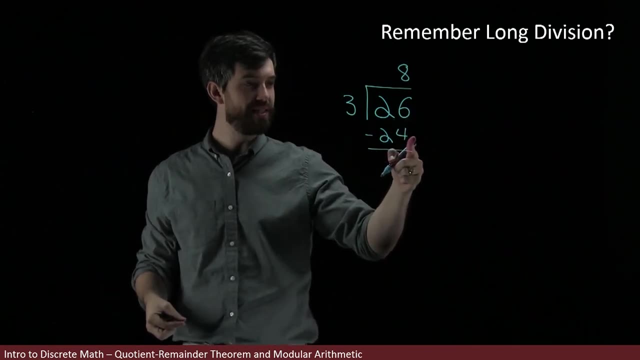 is a number divisible by 3 and as close to 26 as I can get without going bigger than it. And then I would usually come and subtract these things and I'd say 26 minus the 24 is going to be equal to a 2.. 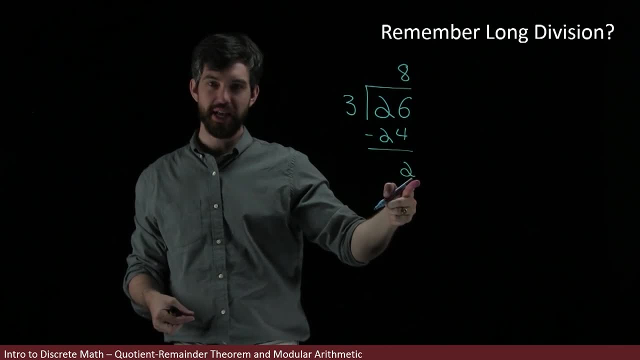 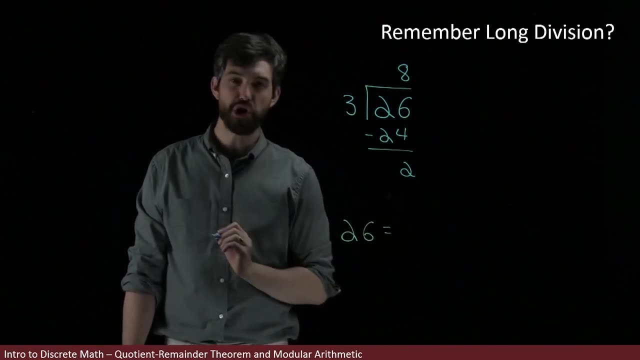 And I had these three different numbers, And the claim is that these three different numbers were going to be related in the following sense: It was that the 26 that I started with was going to be the 3 that I'm trying to divide it by. 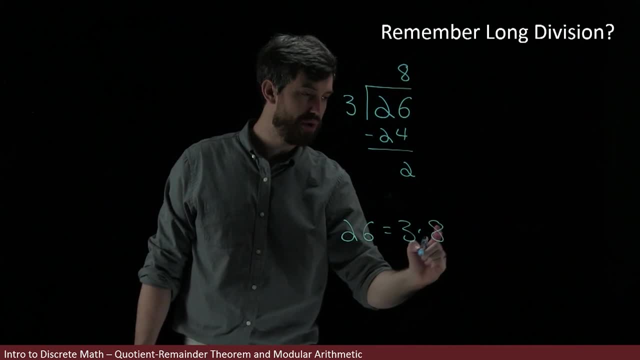 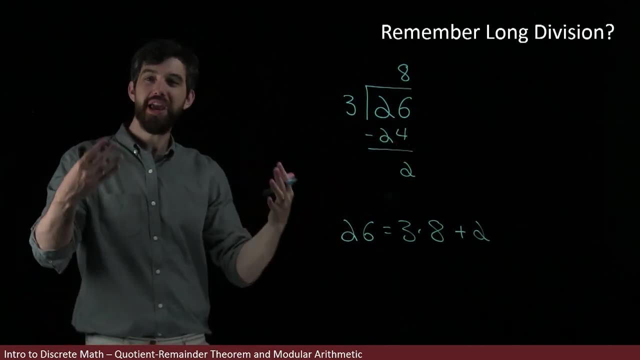 this number up here 3 times 8,, that's the 24, and finally plus 2.. So this sort of whole bunch of symbology was just a way that we could keep track of the steps that we were going, but what our goal was always to say. 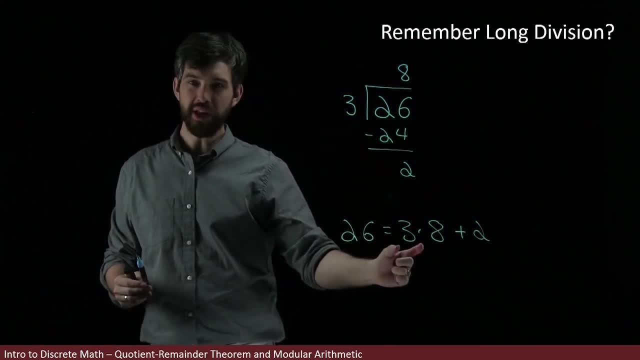 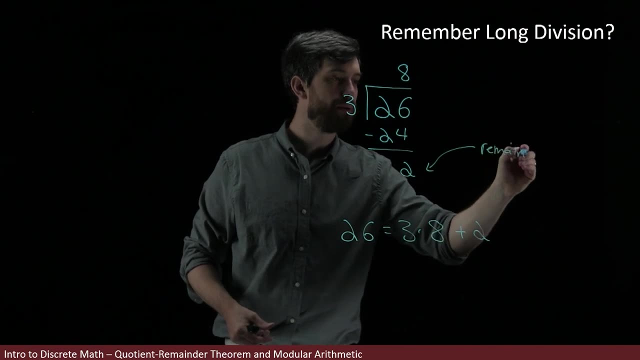 take this 26, write it as a 3 times some other integer, and then I get this 2 here, where the 2 was going to be referred to as the remainder. So this was how our long division worked, but now we want to investigate how 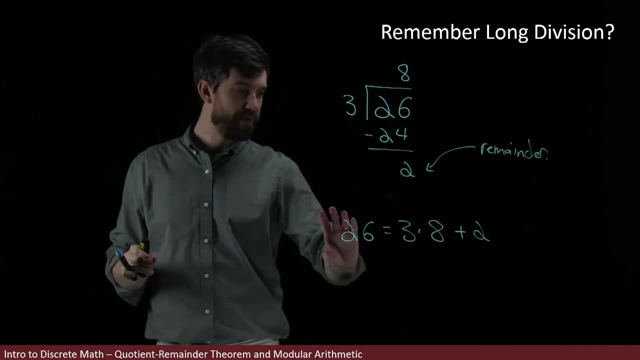 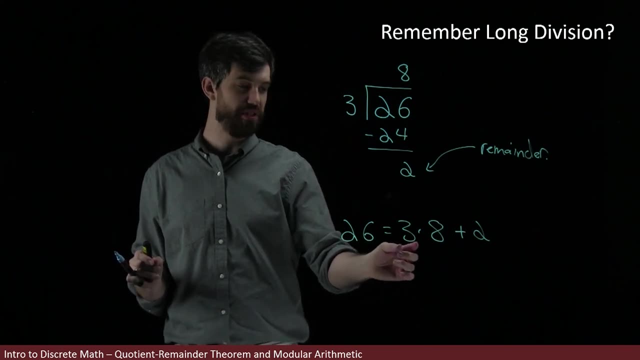 this is going to work formally And I'm going to note that I'm going to particularly like using this bottom equation that we have down here, where we're taking the number that I have and saying that this is equal to the number that I'm dividing it by times. 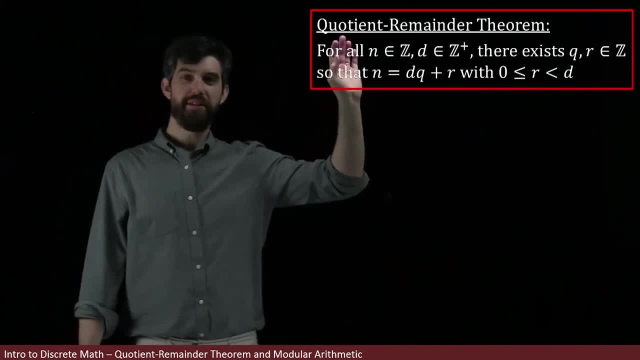 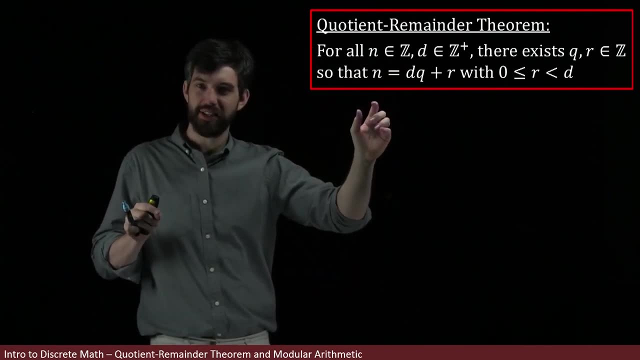 some integer plus a remainder. This funky collection of symbols is called the Quotient Remainder Theorem And basically what the Quotient Remainder Theorem says is long division, that process that we've done many times before, that process actually works. 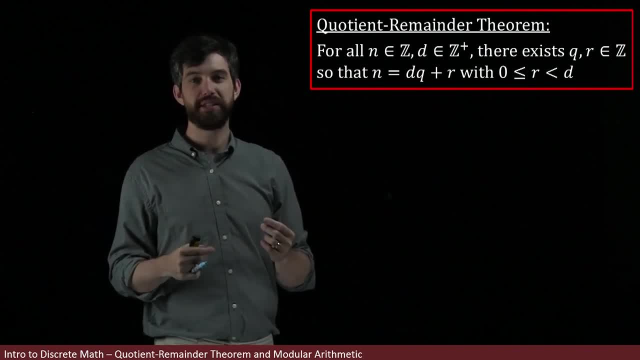 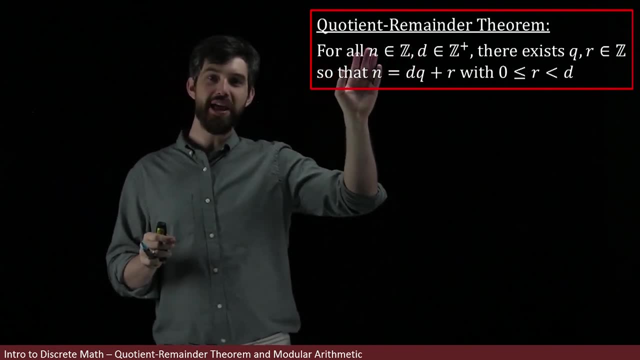 And in fact it always works. In other words, if you have any pair where you begin with some integer n and you divide that integer n by some other integer, that is actually going to be a positive integer. I'm not allowing a division by 0.. 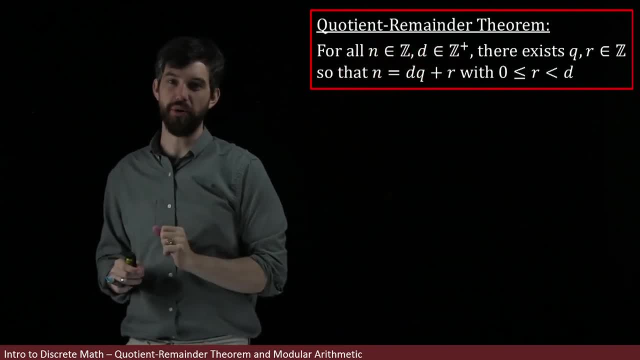 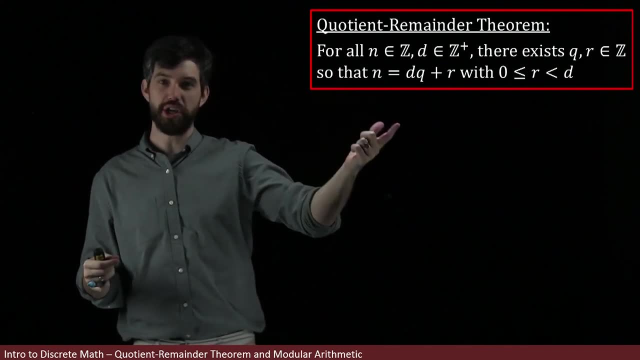 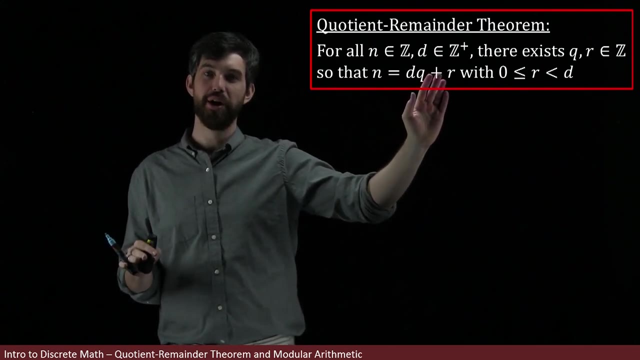 So I've got some n. I'm dividing it by d, which is non-zero. Then we're saying there is a way, as in, there's that remainder and there's this quotient q, where I can go and say that n is written as the divisor d times q. 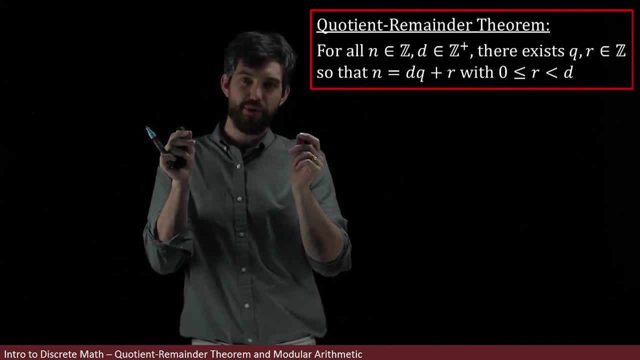 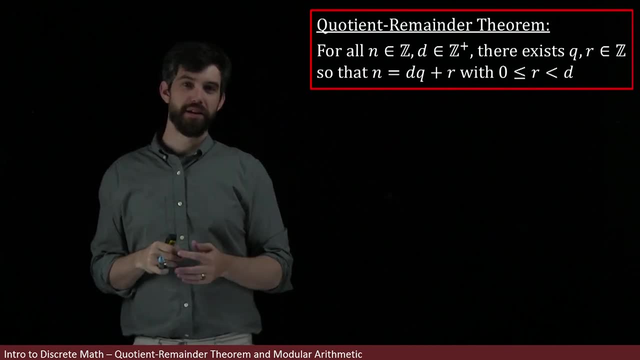 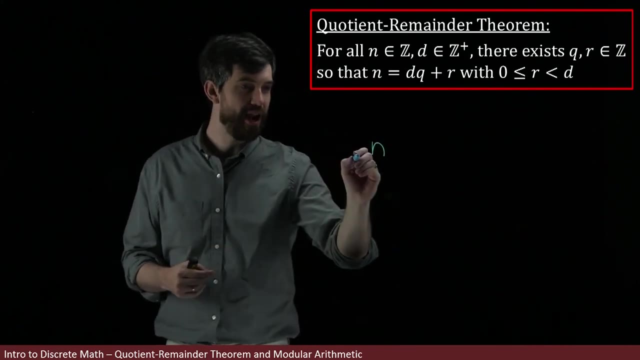 plus this remainder And additionally, that remainder is constrained, that it's somewhere between 0 and the divisor. So let's try to translate this into what we were just saying. The idea would be that if I had some n- and I was trying 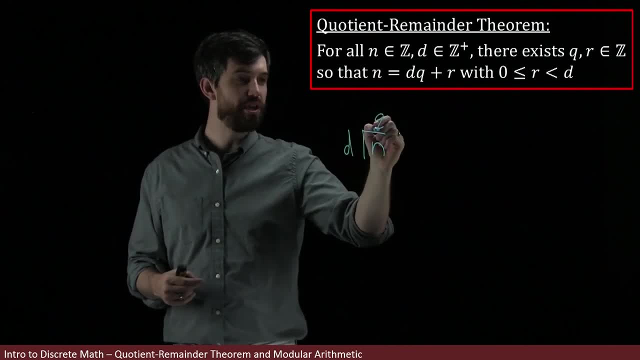 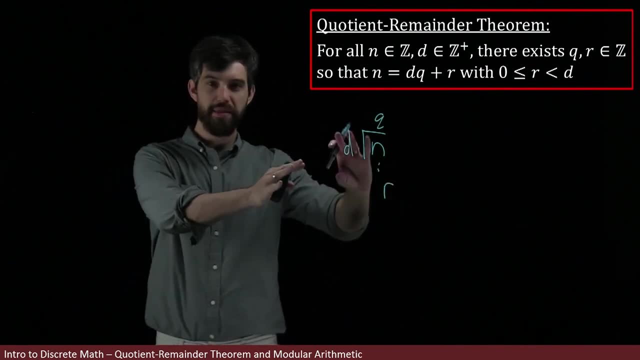 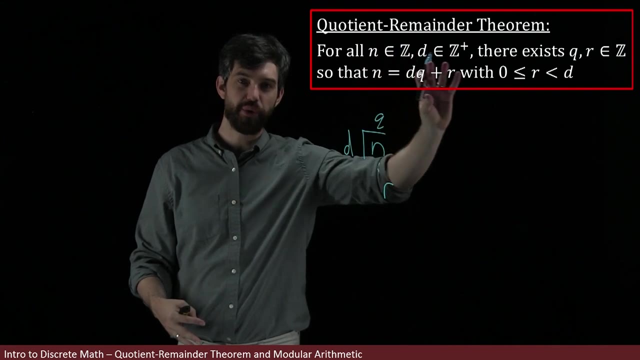 to divide it out by d. I got some q up here and I'd be left with a remainder down here, And then this arrangement of symbols was just sort of one familiar way to collect it. But this is all exactly the same as this arrangement of symbols. 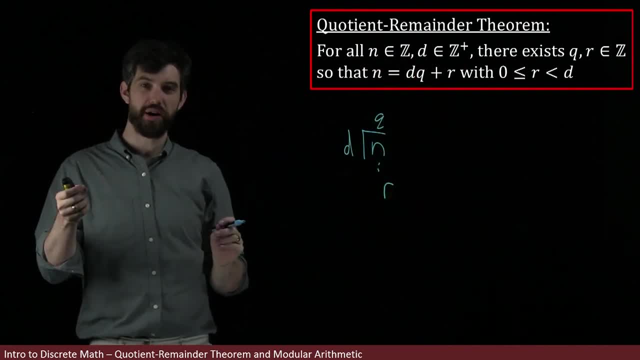 that I have over here. The n is equal to the dq plus the r. Now, while I'm not planning on proving this particular theory, I've got to remember that there's a number of numbers that we need to be able to do. 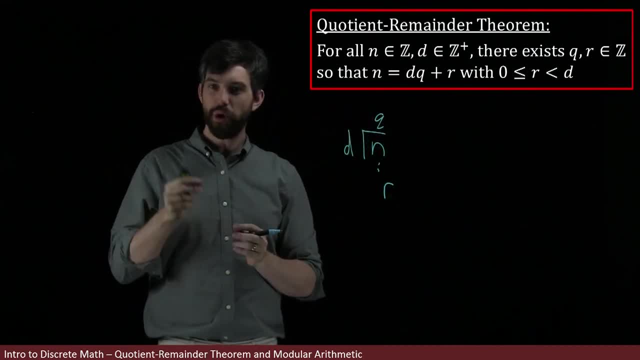 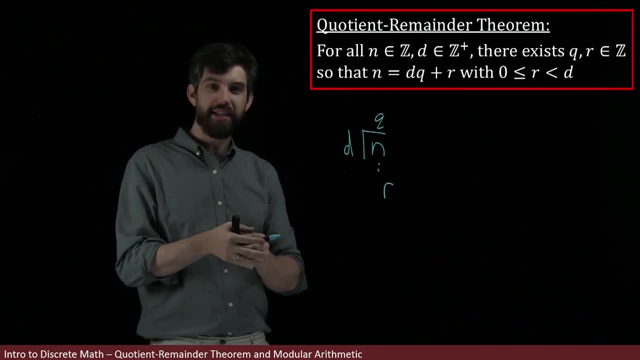 So what I'm doing is I'm going to try and do a simple, particular theorem in this video. it's worth noting that this process that we've had in this past- that was something that we just sort of always went through- is it is actually formalized. 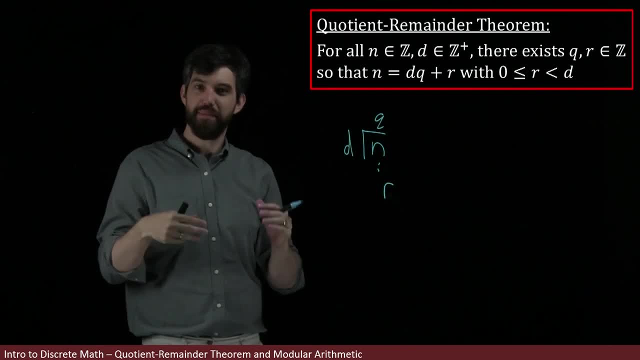 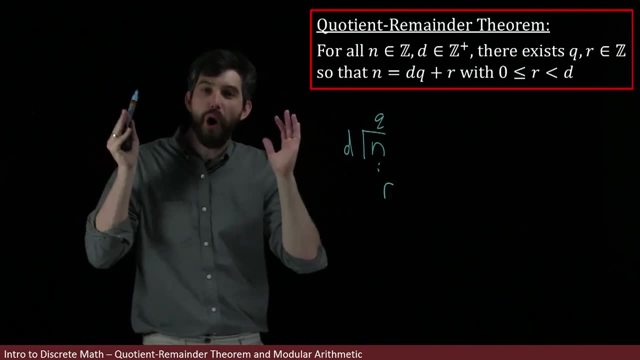 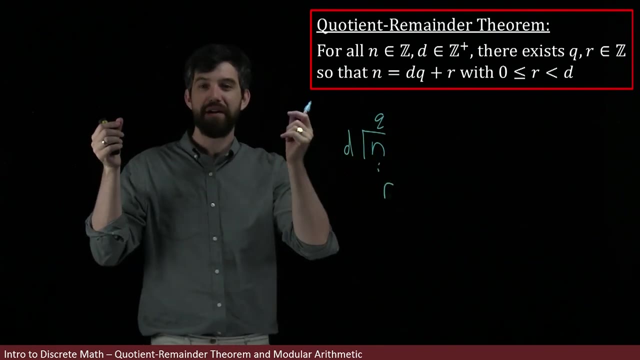 into a proper mathematical theorem, And it's a mathematical theorem that can indeed be proven, And the main takeaway of this theorem is that it always works For all n and d. we're going to be able to write out this relationship between the n and d, where I have this q and where I have this. 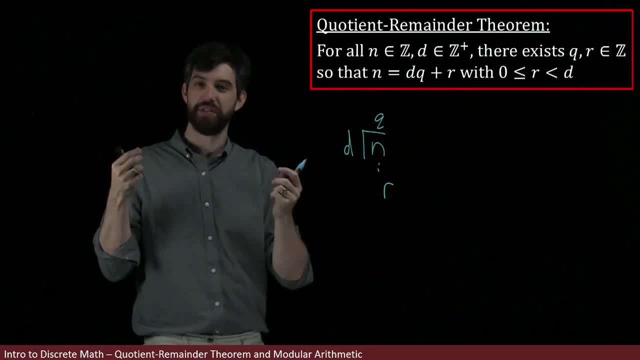 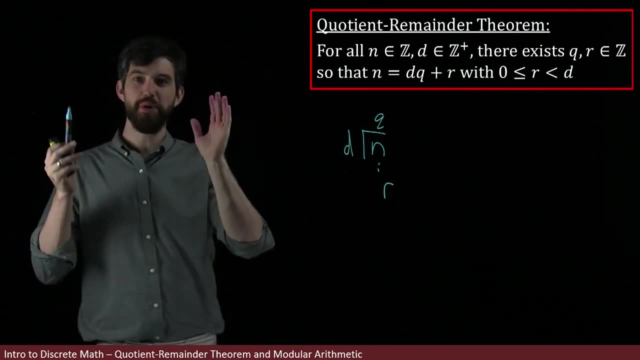 r that fits this particular constraint, so being between the 0 and the d. Now, in some applications, the part that we really care about, the one that we want to focus on, is what this remainder is. That, in some sense, the remainder is the interesting part. 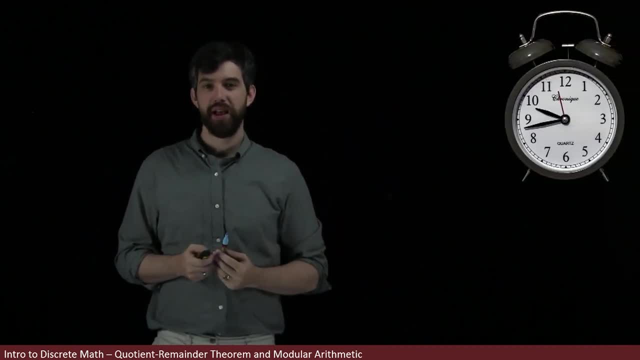 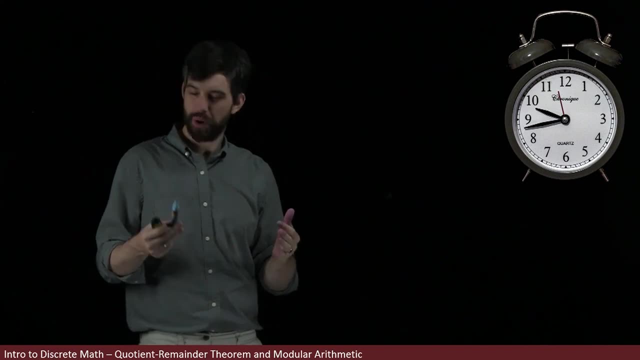 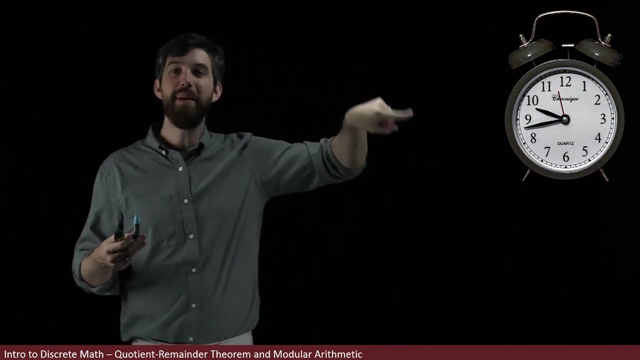 I'll give you an example. Consider a clock. Here I have an analog clock that goes around for 12 hours. This is a form of what we're going to call modular arithmetic, And the idea is this: A clock doesn't tell me how many times it's gone around, It just tells me. 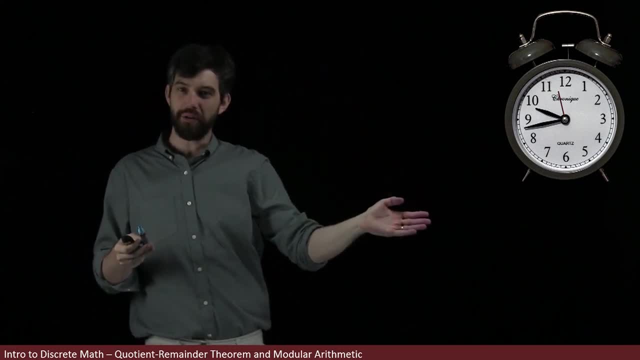 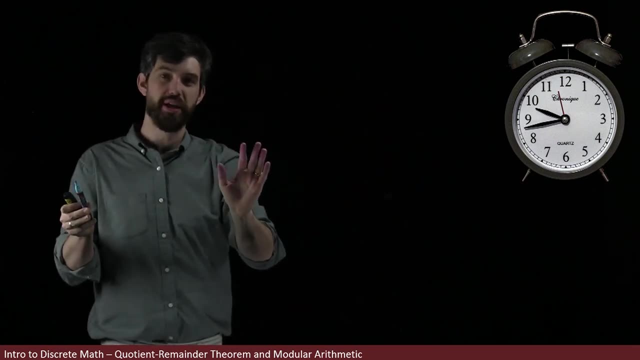 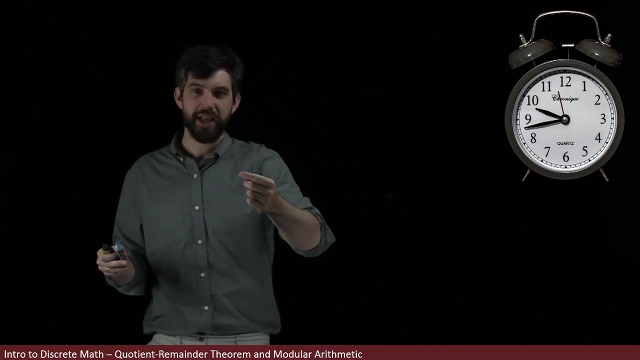 some number between 0 and 12.. It doesn't tell me whether I've gone around the circle like eight times and then ended up at 3 o'clock. It only tells me the 3 o'clock, And what we're going to try to do is pair that idea with only caring about the remainder in the quotient remainder theorem. 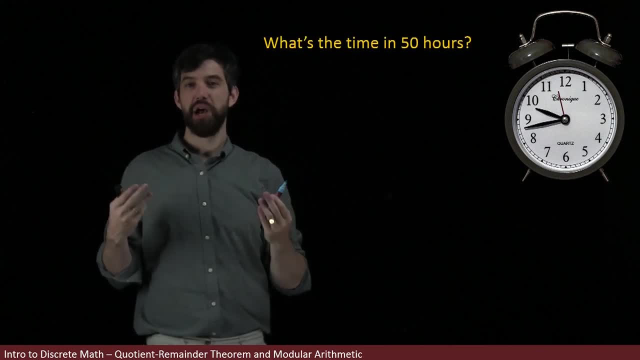 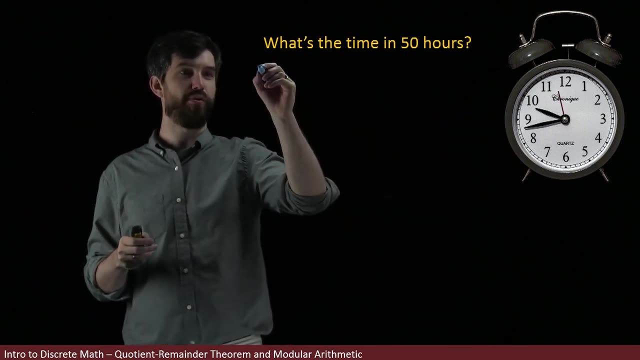 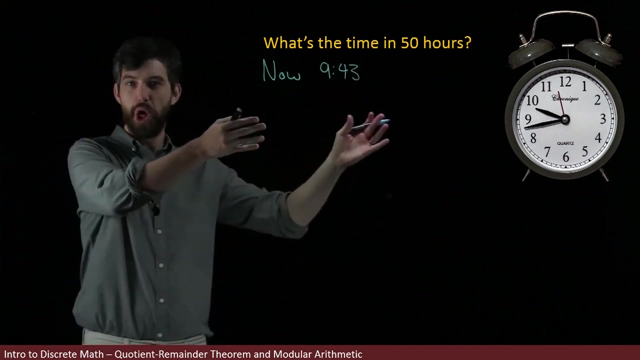 So, for instance, suppose I ask a question like this: What's the time in 50 hours? And if I look at this clock, it looks like we're talking about 943 is where we are right now. So now it's going to be 943.. No, by the way, the clock doesn't. 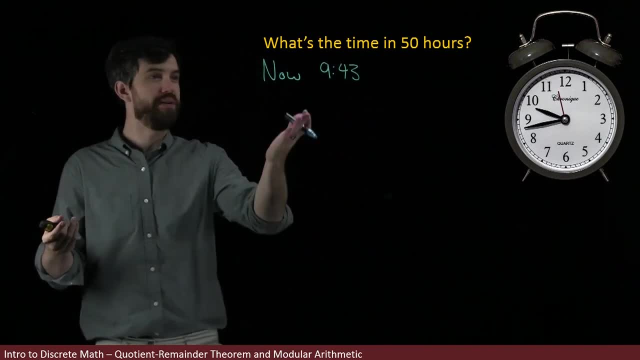 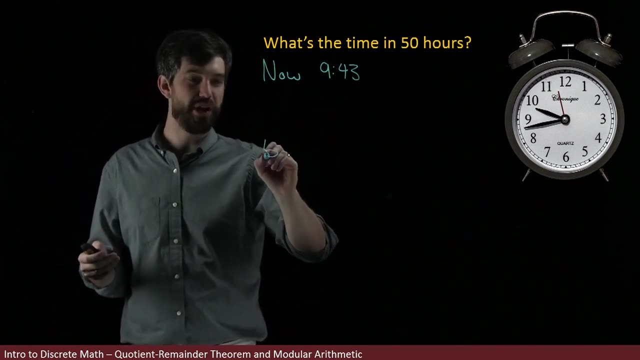 tell me whether it's am or pm either. It just tells me it's some 943.. Now if I then go and I try to like add 50 hours, like I'm going to go 50 hours into the future from this 943, and I want 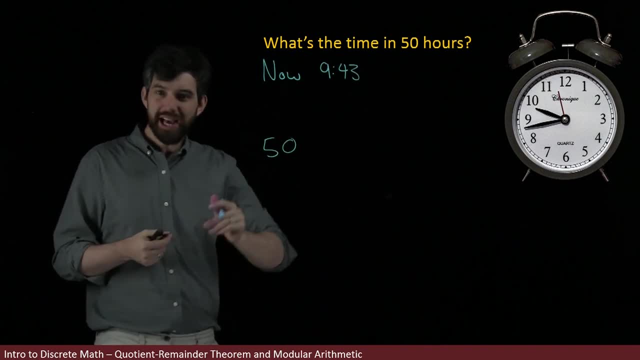 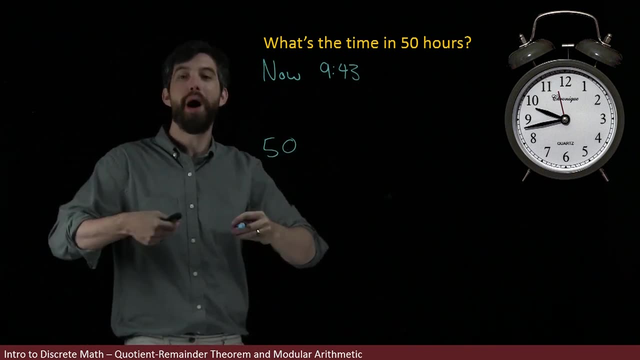 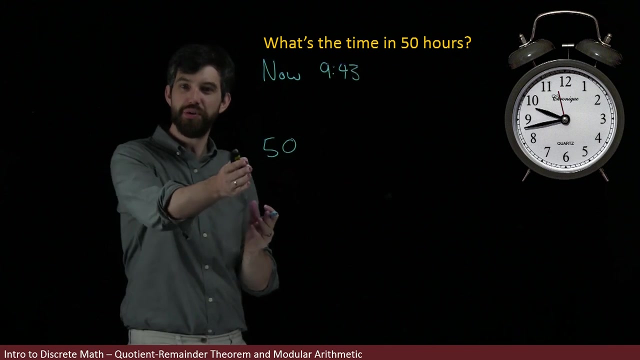 to visit 50 hours from now. Well, because we're dividing out by 12,, like I can't tell the difference between 943 and 12 hours beyond 943, or 24 hours between 943,, this clock will only ever say 943. So what I want to do is sort of divide out by 12.. So I'm going to divide out by 12 here. 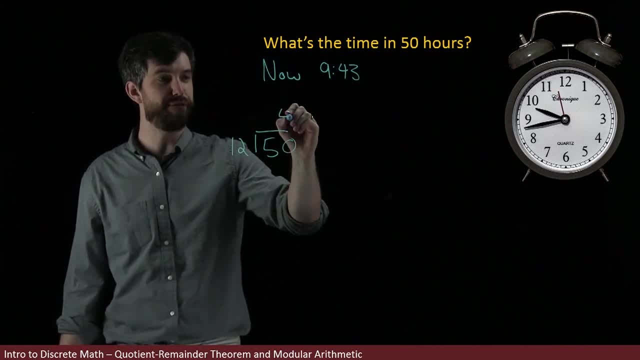 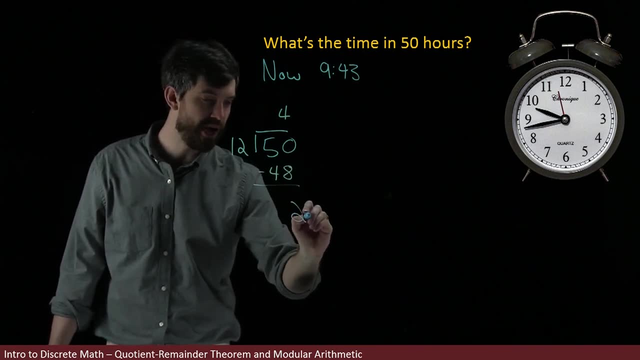 And how does this work? Well, 12 goes into 50. four times That leaves me with 48. And if I subtract 50 from 48, that gives me a remainder of two hours. So in other words, if I'm 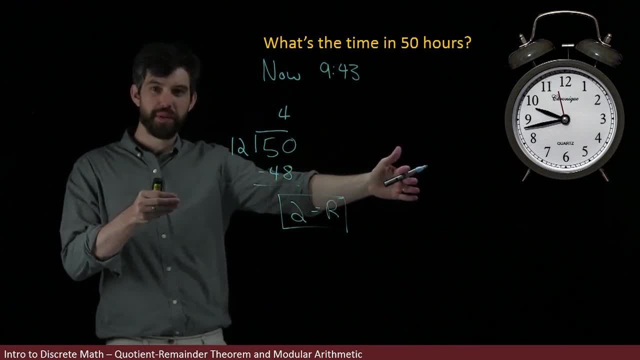 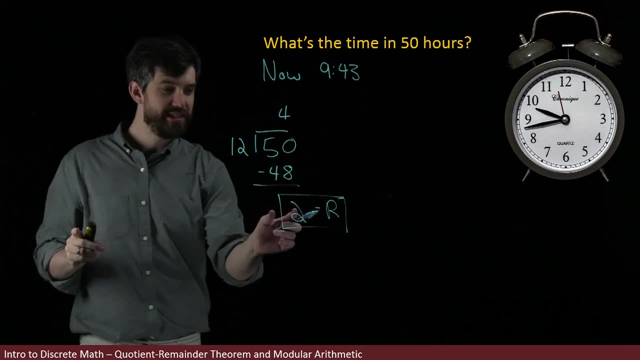 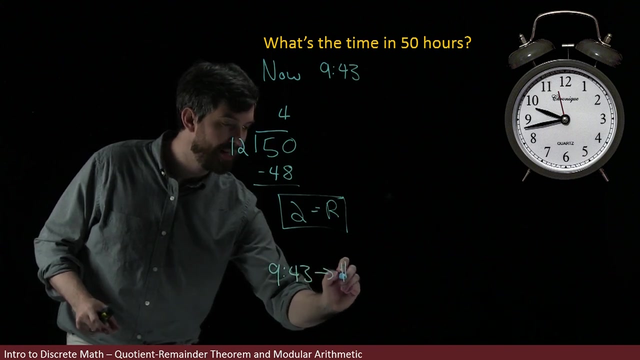 going to advance from 943 50 hours into the future. the first 48 hours is just me wrapping around the clock and getting back up to 943. But what matters is the extra two hours in the remainder. In other words, I go from 943 to 1143, where I've added the two hours. 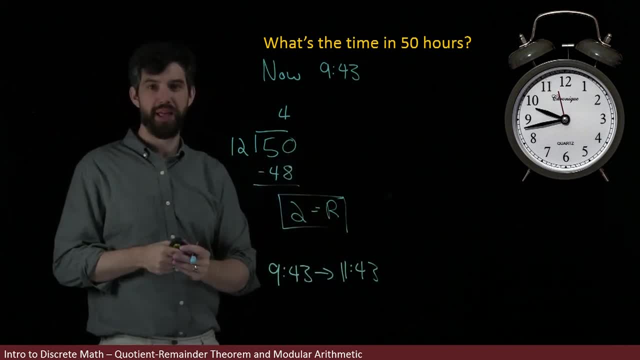 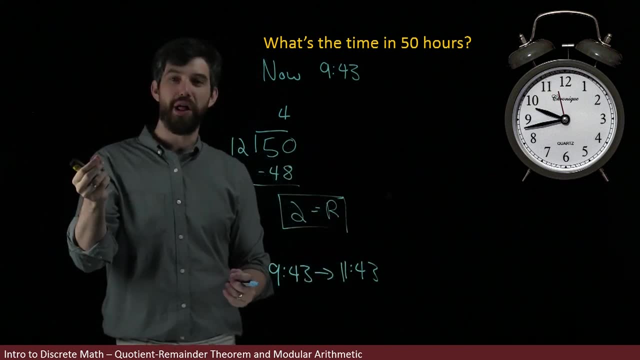 The fact that I've also added 48 just isn't detectable in any way. So this is referred to giving me the value of this modulo 12, where we don't keep track of how many times we go around 12 hours, We only keep track of how the remainder changes, the shift of two hours extra from the 943. 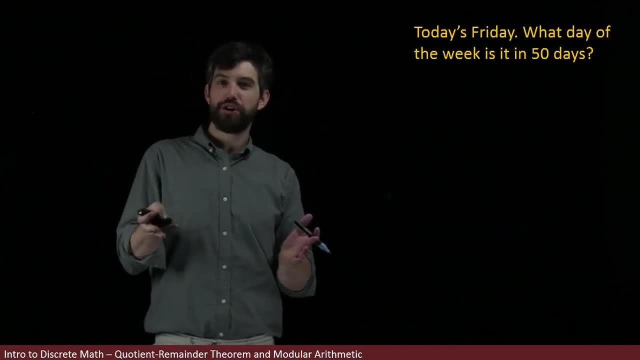 to 1143.. We also use modular arithmetic when it comes to days of the week. Days of the week are something that repeat every seven days, And so I can ask a question like: if today is Friday, what day of the week is it in 50 days? 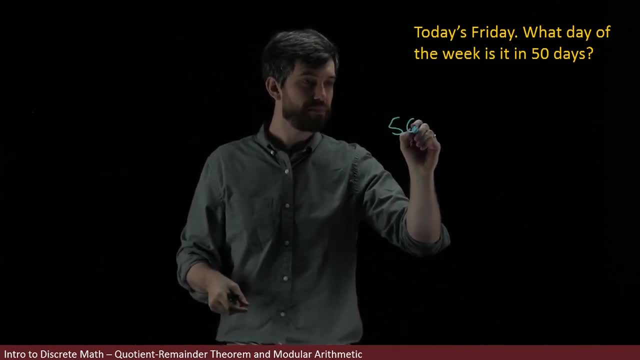 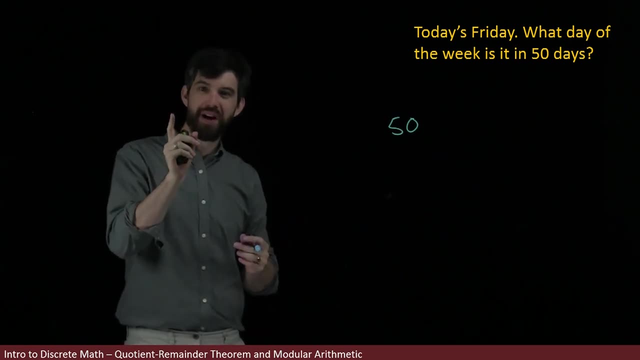 And I'm going to do much the same sort of process. I'm going to take my 50.. Instead of dividing it by 12,, though, or taking it, as they say, modulo 12,, I'm going to take it, dividing it out by seven. 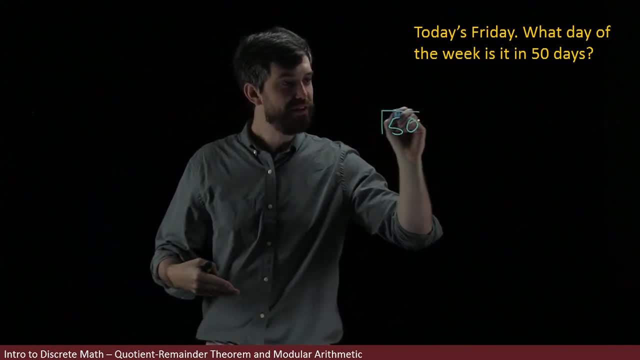 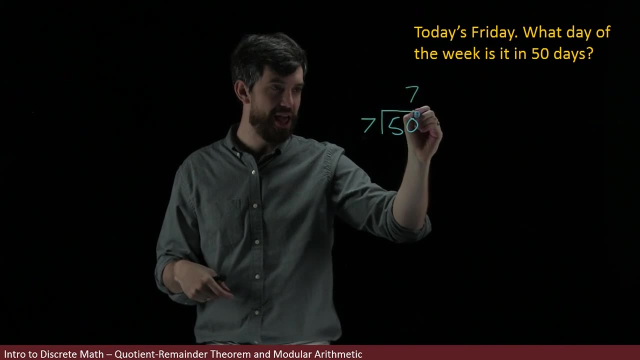 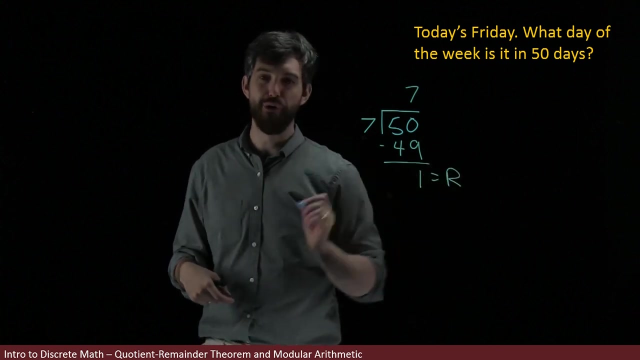 because there's seven days in the week. So let me divide this by seven, And then I know that seven takes me with 49. And if I subtract the 49, I'm going to get a remainder of one. And so what? I? 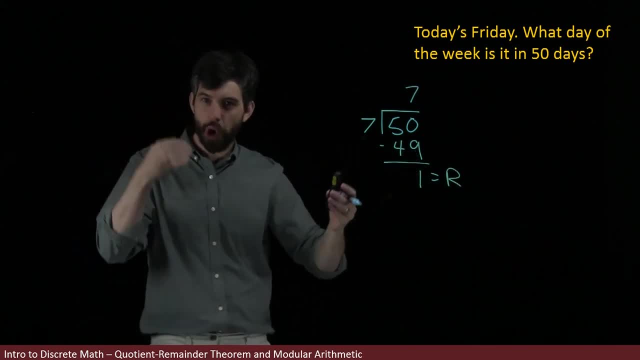 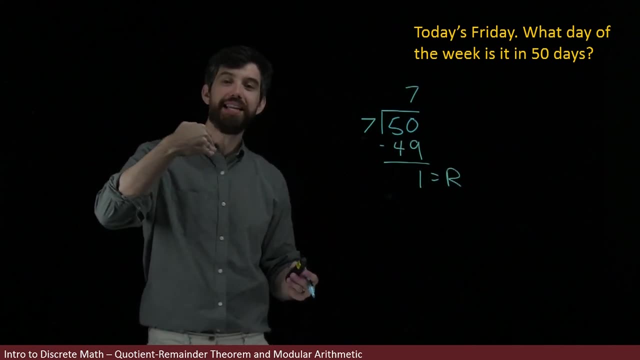 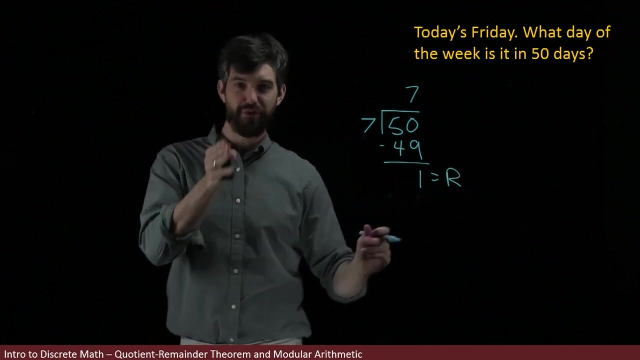 think about this is that if I'm advancing my 50 days and I start on Friday after seven days, I'm back on Friday After 14 days. I'm back on Friday After 49 days, because that's divisible by seven, I'm back on Friday as well, And then I have a remainder of one, which takes me from. 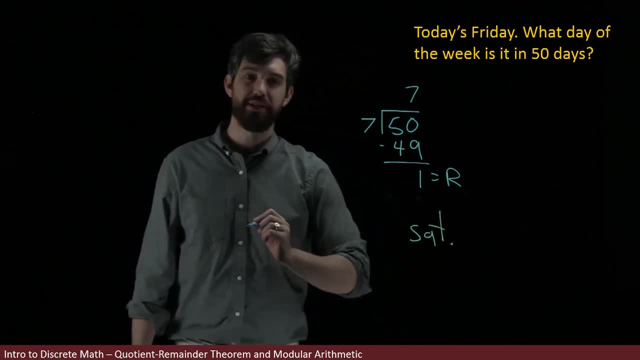 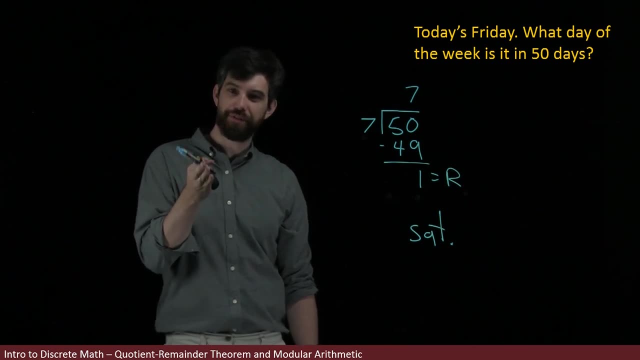 Friday to Saturday. So where do I end up with? I end up being on Saturday, So this kind of modular arithmetic occurs in all sorts of different places, but I want to be able to define it precisely, So I've brought back up my quotient. 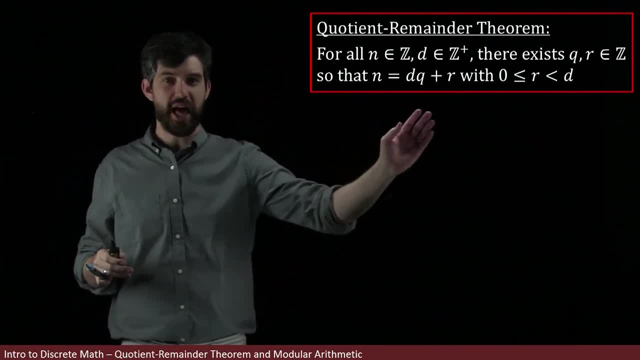 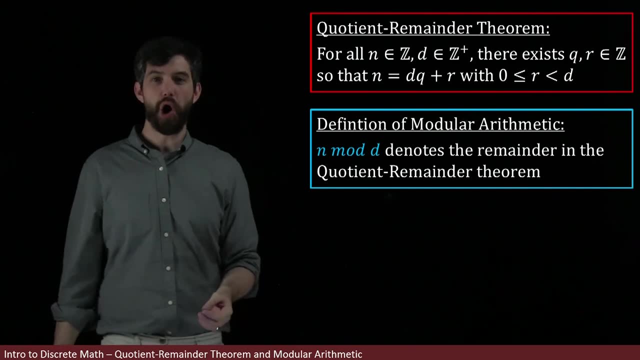 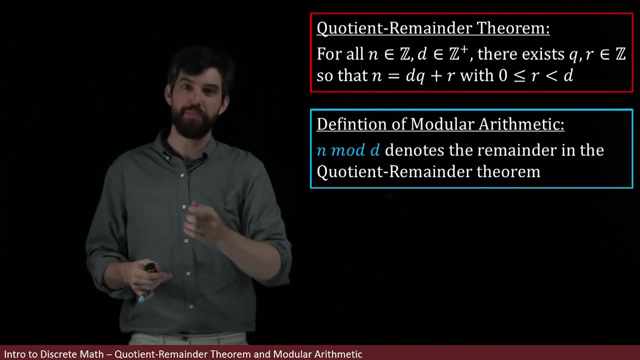 remainder theorem And the idea with modular arithmetic is that I'm only caring just about the R. So here is my precise definition. The terminology is always going to be n mod d, So in this case n is the big number that I have- the 50 in my previous. 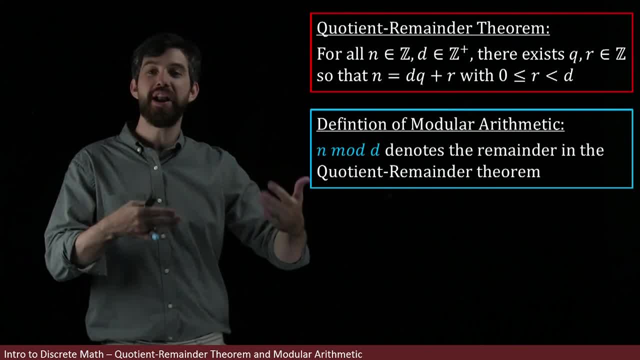 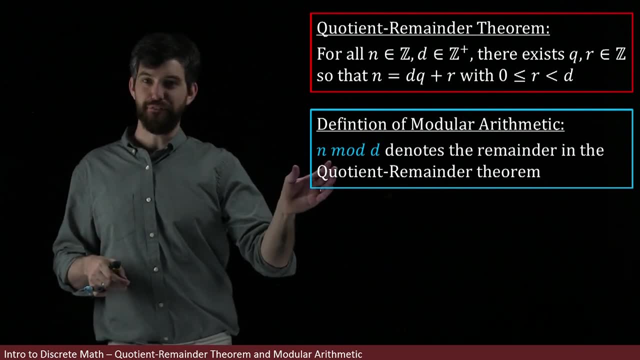 example d represents what I'm sort of dividing it into. So it was the 12 in the case of the clock or the 7 in the case of the days of the week. So I might say something like 50 mod 7.. And what we?